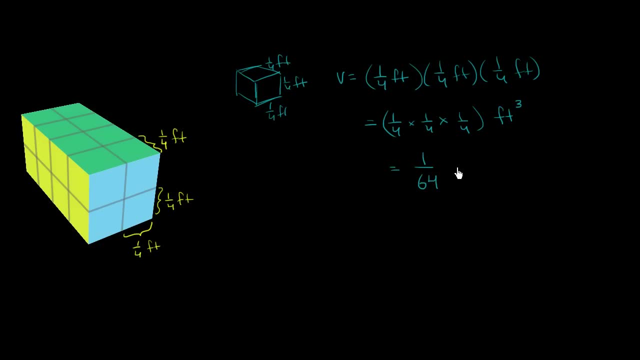 So this is going to be 1 over 64 cubic feet. Cubic feet, or 1 64th of a cubic foot, That's the volume of each of these unit cubes. Now, how many of them are there? Well, you could view them as kind of these two layers. 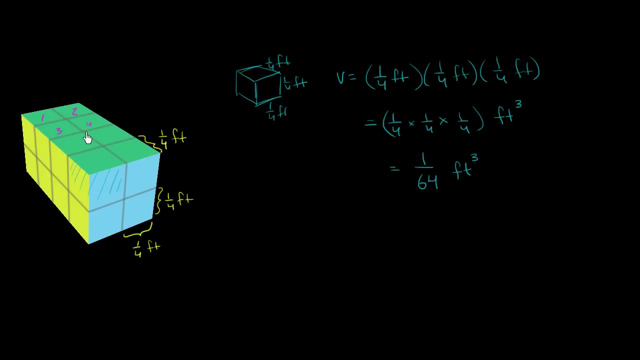 The first layer has 1,, 2,, 3,, 4,, 5,, 6,, 7, 8.. That's this first layer right over here, And then we have the second layer down here, which would be another 8.. 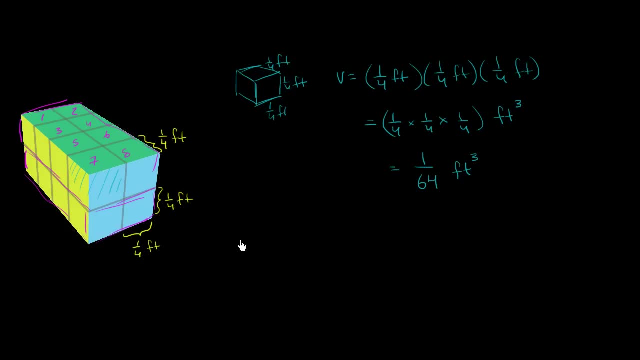 So it's going to be 8 plus 8, or 16.. So the total volume here is going to be 16 times 1 64th of a cubic foot, which is going to be equal to 16 over 64 cubic feet, which. 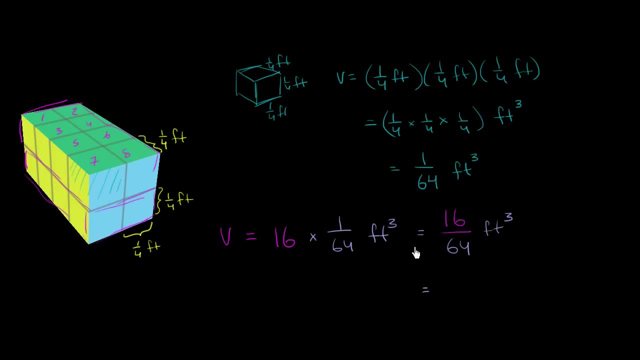 is the same thing. 16 64ths is the same thing as 1 fourth. Divide the numerator and the denominator by 16.. This is the same thing as 1 fourth of a cubic foot, and that's our volume. Now, there's other ways that you could have done this. 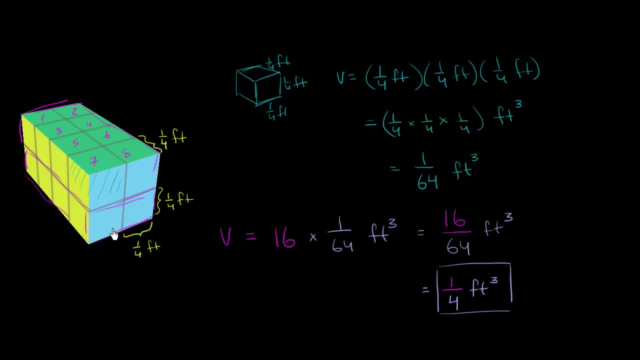 You could have just thought about the dimensions of the length, the width and the height. The width right over here is going to be 2 times 1 fourth feet, which is equal to 1 half of a foot. The height here is the same thing. 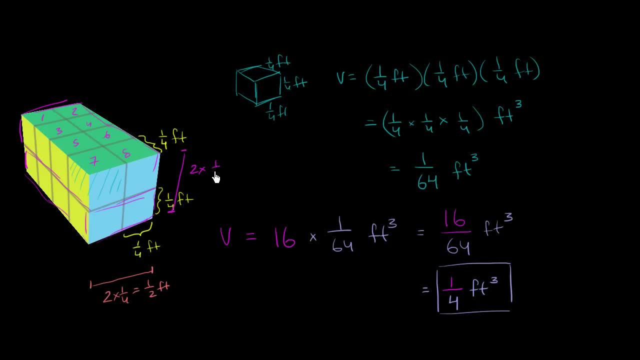 It's 2 times, So it's going to be 2.. 2 times 1 fourth of a foot, which is equal to 2 fourths or 1 half of a foot, And then the length here is 4 times 1 fourth of a foot. 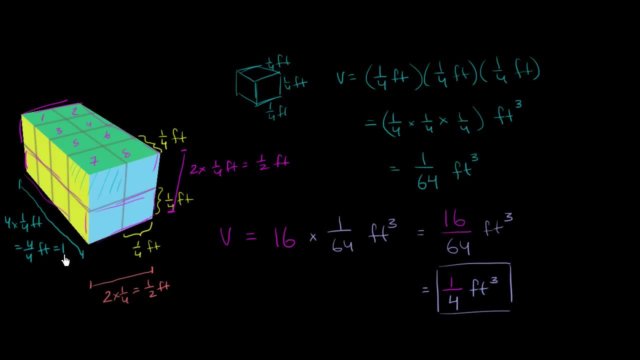 Well, that's equal to 4 fourths of a foot, which is equal to 1 foot. So to figure out the volume, we could multiply the length times the width, The length times the width times the height. And these little dots here, these aren't decimals.